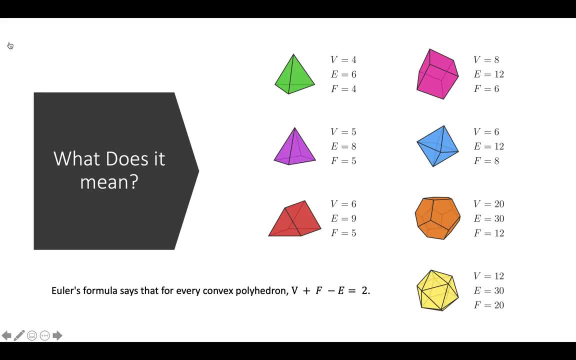 that it has a formula for polyhedra, And we'll notice that it has a formula for polyhedra. And we'll notice that it has a formula for polyhedra And we'll notice that it has a formula for 8 vertexes, 12 edges and 6 faces. Well, if you just follow the equation blindly and you add 8 to 6, 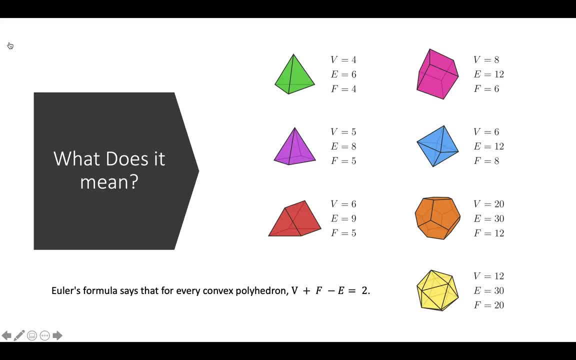 8 vertexes, 12 edges and 6 faces. Well, if you just follow the equation blindly and you add 8 to 6 4texes plus faces, you get 14,. minus off the edges: 2, and you get 2.. And that's not a coincidence. 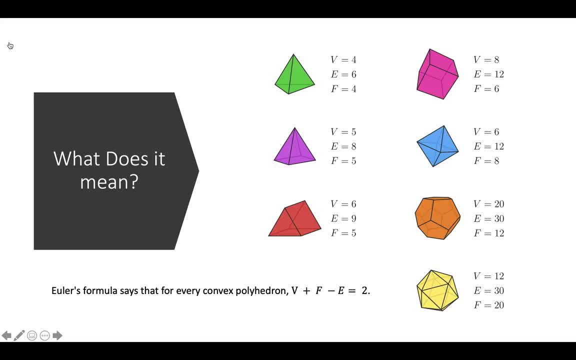 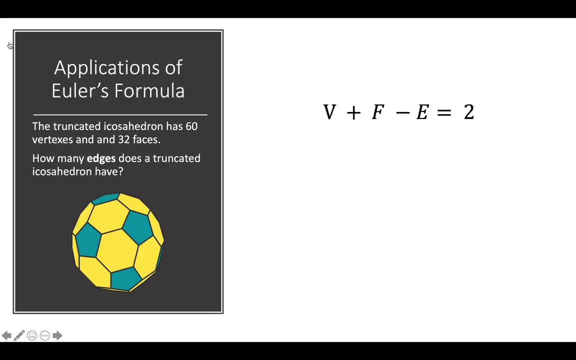 And that's true for any convex polyhedra like the one shown here, which is a pretty astounding fact. Applications of Euler's formula. So this is a very simple example, just just to get us warmed up and to see the usefulness of the formula. So we're. 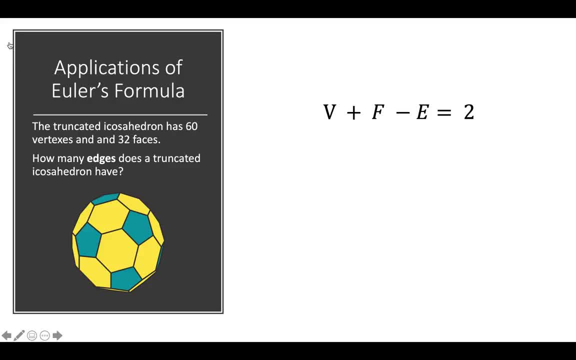 presented a polyhedra. we're told how that it has 60 vertexes and 32 faces, and they want to know how many edges it has. So one way we could do this is count it, but you can imagine how awful that would be. with such a complex shape, You would 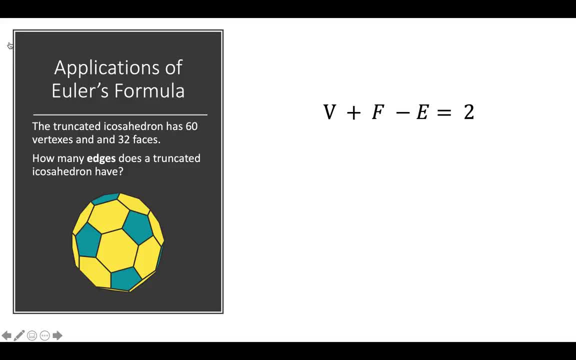 lose track, you might over count and have to restart. you get an odd number and you wonder why you have to restart. So instead we'll just plug it into Euler's fuller formula, because we have all the information we need. all we're missing is: 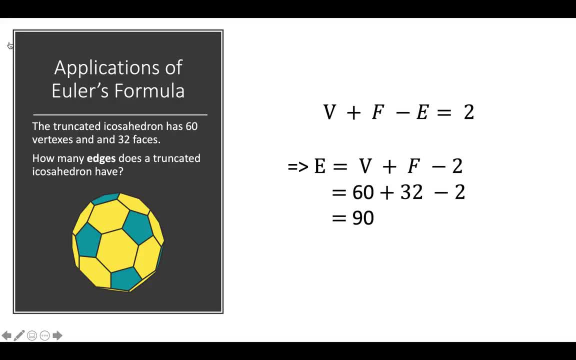 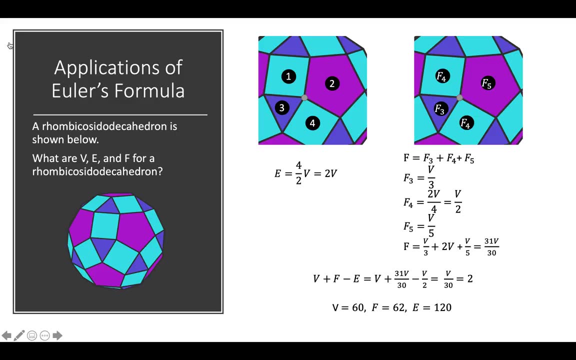 the edges, Plugging it into the formula. it's pretty straightforward: E, you solve for E, plug in V for 60,, F for 32, minus 2 and you get 90.. Moving on to a more challenging example, in this example we're given a polyhedra, but we're not. 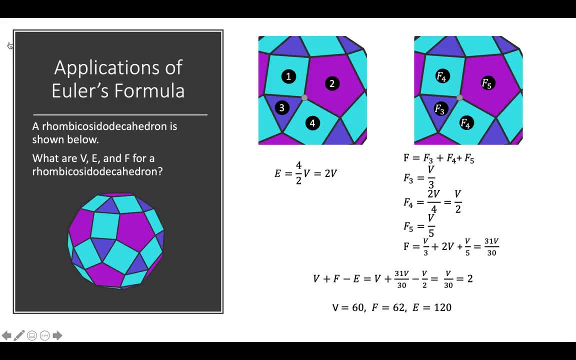 given any information, we have to deduce it all ourselves. we're just given a picture. So how do we attack this? We notice that every vertex has an odd number and we want to know how many edges we have. So every vertex is identical. What I mean by identical is every. 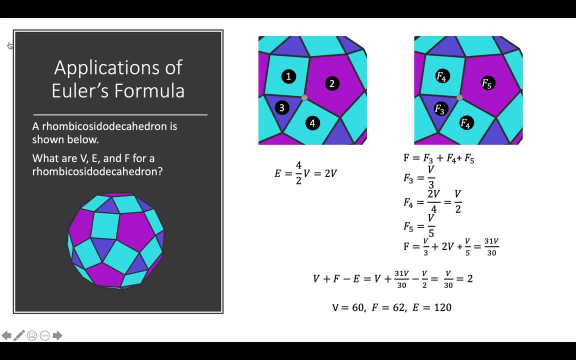 vertex has a hexagon, two squares and a triangle on it, So we could use that fact to get our edges as a function of vertexes and our faces as a function of vertexes. So let's start out with edges. So I have this picture with the numbers. 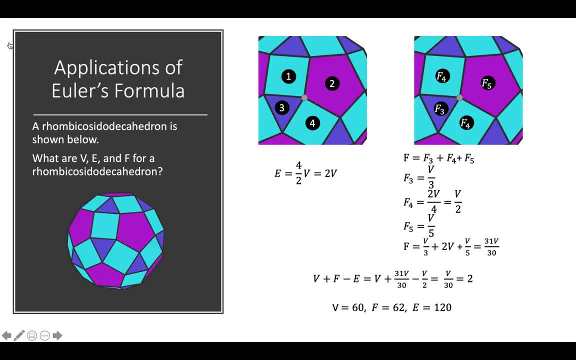 1,, 2,, 3 and 4 on it. This picture is trying to show that every vertex has four edges on it, So edges equals four times the vertexes. but every edge has two vertexes attached to it, So we have to divide by two to not over count, which gives us E equals 2V. 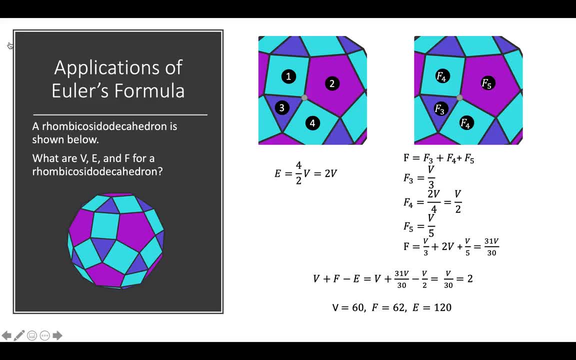 We need to do the same thing for the faces. Faces are a little bit more complicated. we're gonna have to break it up to different cases. So F3 represents a triangle, F4 a square and F5 a hexagon. Notice that if we add up all the squares, 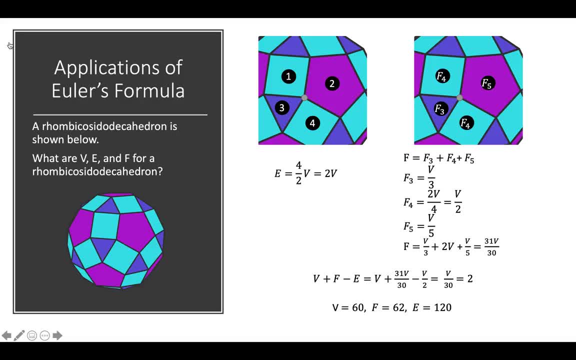 triangles and hexagons, we'll have the total number of faces. So let's start with triangle. Notice that every vertex has one triangle attached to it, but every triangle has three vertexes. So V divided by three will give us the number of triangle faces. Moving on to squares, Notice that every vertex has three. 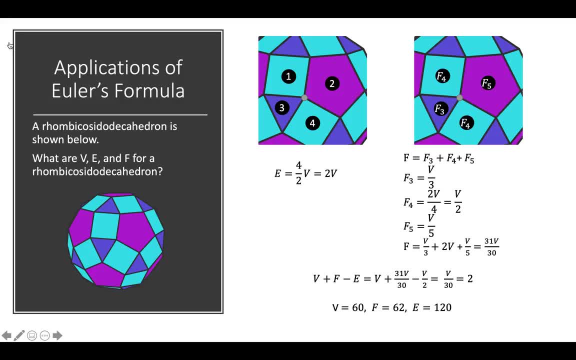 squares attached to it, but every square has four vertexes. So 2V divided by four, Simplifying, we have half as many squares as we do vertexes. Finally, moving on to the hexagon, Every vertex has one hexagon, but every hexagon has five. 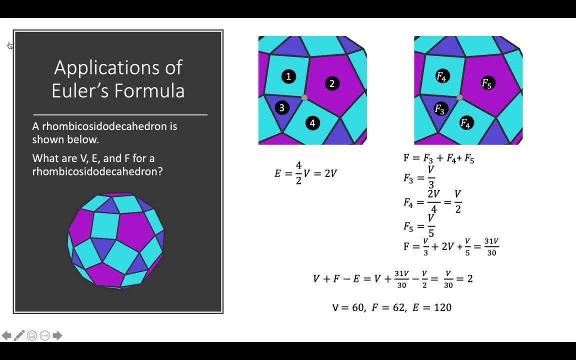 vertexes, So V divided by five. So then we just plug that into our equation for F and we get that F equals 31V over 30.. Okay, so now this is where Euler's formula comes in. So we have V plus F, minus E. just makes our substitutions, because we 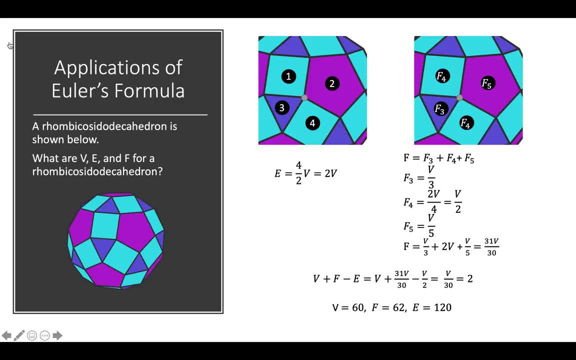 know what E is in terms of V and we know what F is in terms of V. We simplify: we get V over 30 equals 2.. Multiplying across, we get V equals 60. But we have E as a function of V, so we just plug 60 in for. 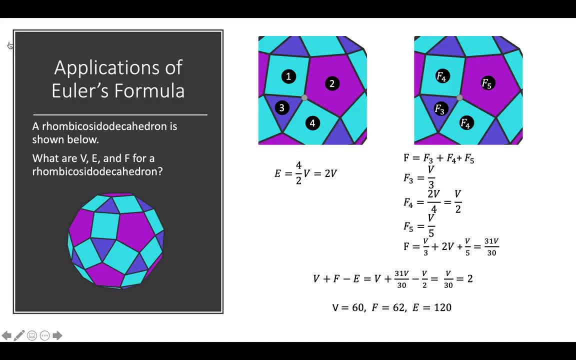 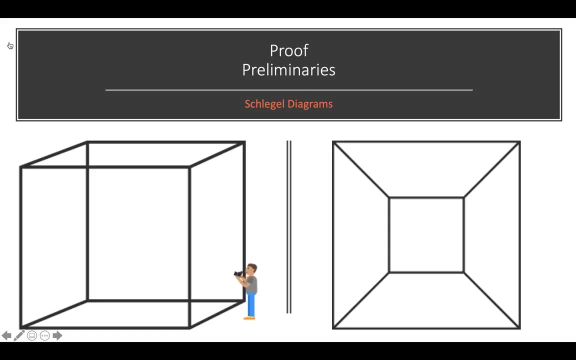 E of V, and that's 2 times 60, which is 120.. So we have 120 edges And the same thing for faces. 31 times 60, divided by 30, equals 62.. Moving on to proof preliminaries, what we're going to need to know to dive into the proof for 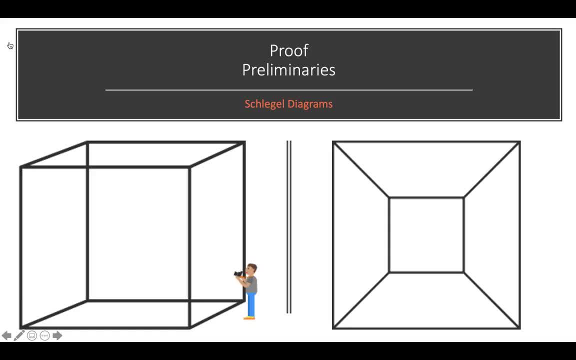 Euler's formula is something called Schlegel diagrams, And you can think of a Schlegel diagram as what something would look like if you took a picture of a polyhedra in front of one of the faces. So on the left we have the picture of somebody taking a picture and on the 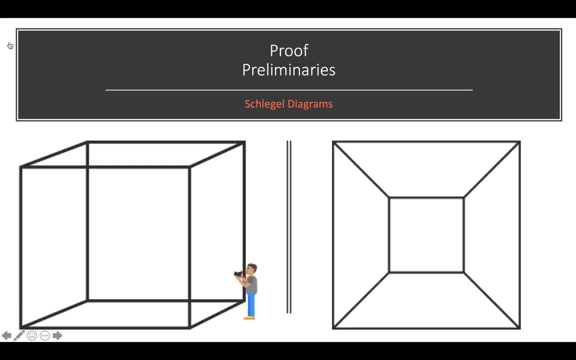 right, we have the Schlegel diagram, what it would look like, And you'll notice that it's nothing but a graph, with some edges and some nodes. This is a very useful way of representing polyhedra. Schlegel diagrams are useful because 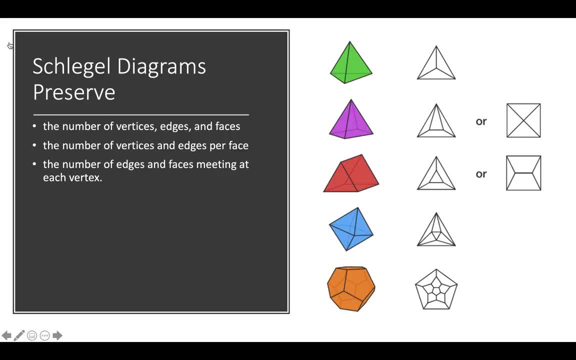 they preserve relevant information about the polyhedra And they're easy to look at, very easy to see all the information in one place. So what do they preserve? They preserve the number of vertices, edges and faces. They also preserve the number of vertices and edges per face. 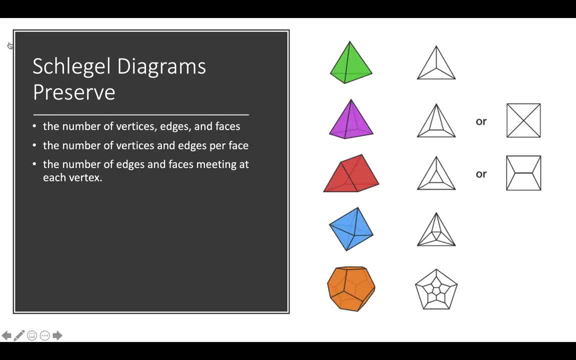 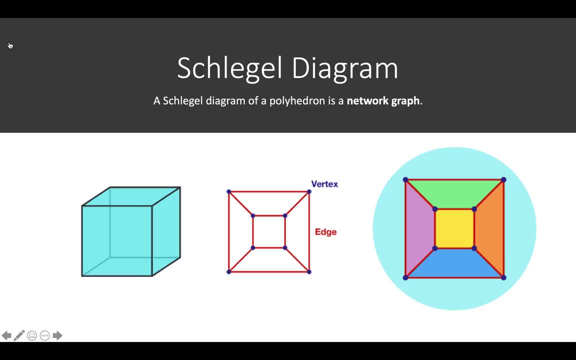 as well as the number of edges and faces meeting at each vertices. So how do we read Schlegel diagrams? Well, Schlegel diagrams is nothing more than a network graph, and you can think of the edge of this graph as the edge of the polyhedra. 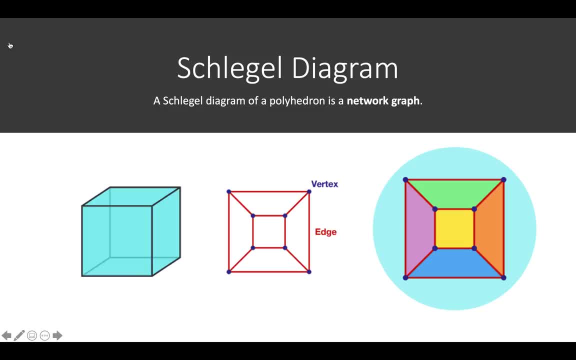 the node of the graph as the vertex of the polyhedra, and then the regions as the faces. So on the far right image you'll notice the blue circle That represents the face closest to the cameraman. in the cameraman analogy, The yellow would be the one furthest away, and so on and so. 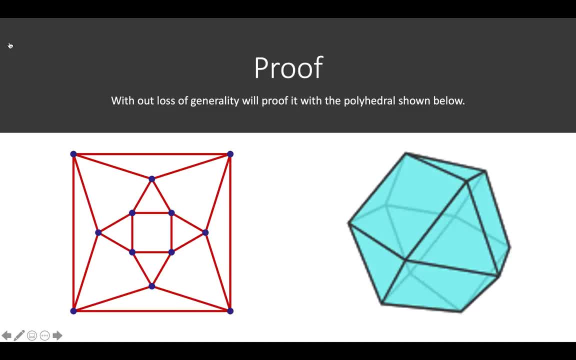 forth. We now have the tools necessary to start attacking the proof of Euler's formula. We're going to do it on a specific example, but it's going to be very, very easy to see that this generalizes very nicely to any polyhedra. So the polyhedra is on. 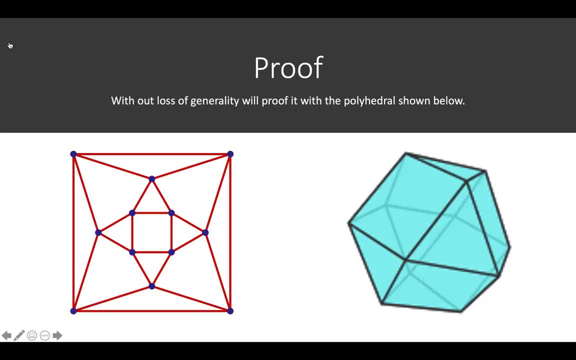 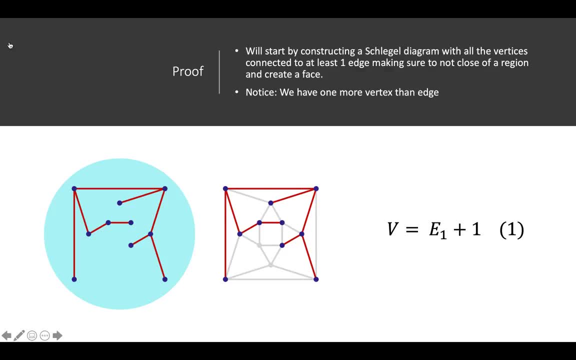 the right and on the left is the graph representation of the polyhedra we're going to be using for the proof. We begin the proof by constructing a partial Schlegel diagram. We connect every vertice with an edge, but we make sure that while we're doing this, 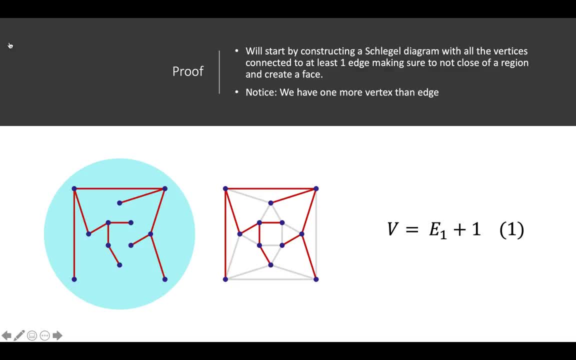 we don't enclose any regions, so we don't want to create any faces, And you'll notice that the first edge we create has two vertices. Then after that every edge comes with an additional vertice until we get to the end. And so if we call all the edges at the end, E1,. 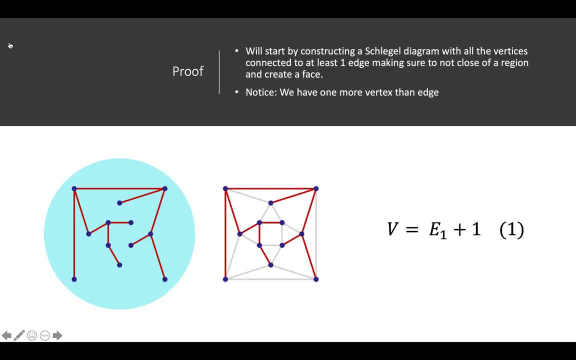 then the vertices equals E1 plus 1, because at the start we have one more vertice than edge and then we just keep adding edges until we get all the vertices. We'll call this equation 1, and it will be useful later on. 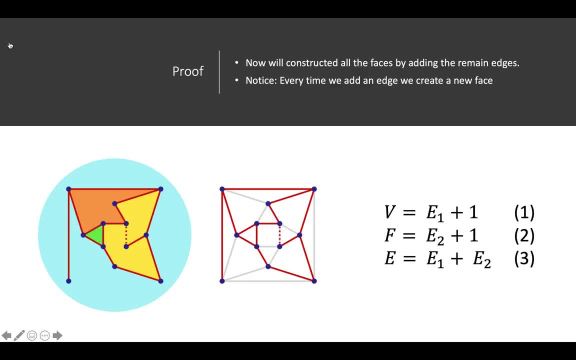 Now we're going to use our partially constructed Schlegel diagram and the remaining edges that we haven't filled in to try to figure out how many faces we have in terms of how many edges we haven't filled in. So what we need to notice is that, starting from 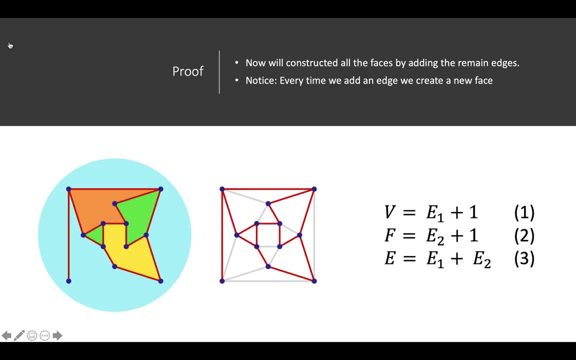 our partial Schlegel diagram. as soon as we add one more edge, we create a region. Remember, regions are like a one-to-one correspondence with faces. So every time we add an edge we're adding a face. But we started out the Schlegel diagram with one face, the blue face. Then we add: 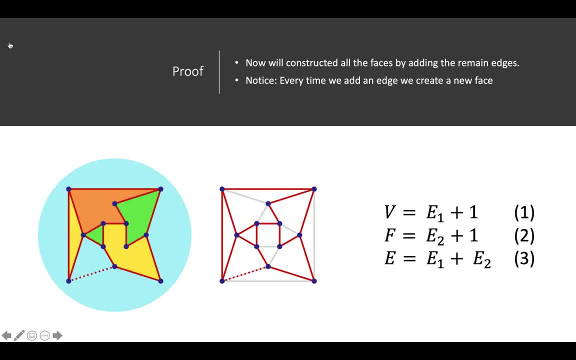 we get another face and we keep adding edges. We add up E2 edges. Every time we add an edge, we add a face. So faces equals E2 plus the initial face that we started with. So this is equation 2, and then we have equation 3, which is nothing more than noticing. 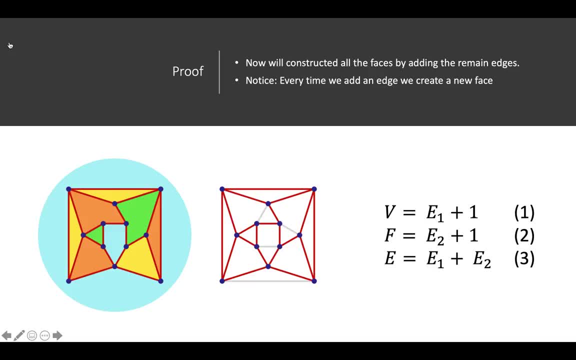 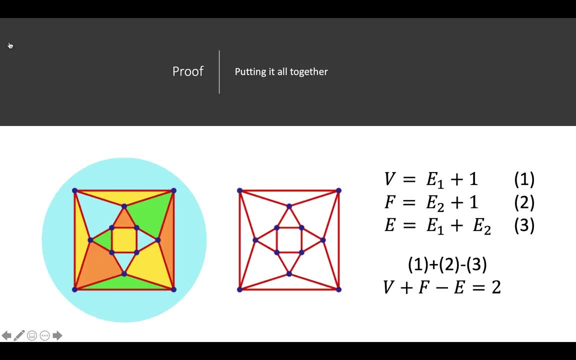 that the total edges was the edges from our initial partial Schlegel diagram, plus the ones we just filled in to create the faces. We now have everything we need to complete our proof. All we need to do is create a linear combination of these equations to construct Euler's formula. So notice that we have. 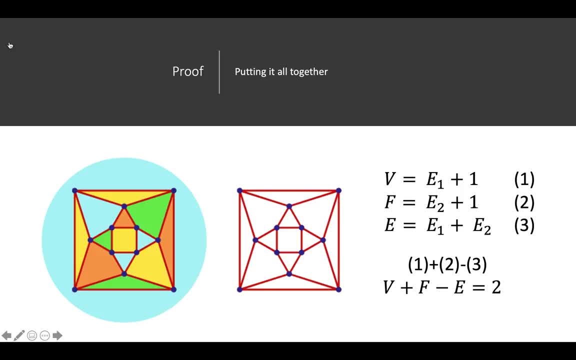 V for equation 1, F for equation 2, and E for equation 3.. So it might be natural to just add equation 1 and 2, V plus F and then minus equation 3, E. And sure enough, when you do that, E1 and E2. 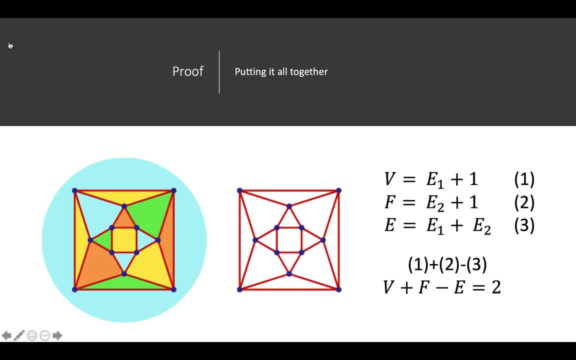 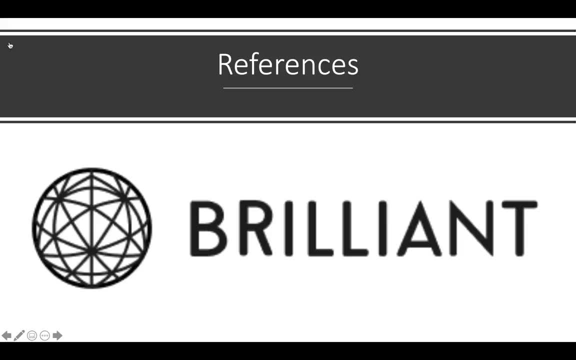 cancel out and you're left with v plus f minus e equals two, aka euler's formula. the only resource i used to create this presentation was brilliantcom. that's where all the images come from and the animations. it's a great resource. i recommend you guys check it out if you want. 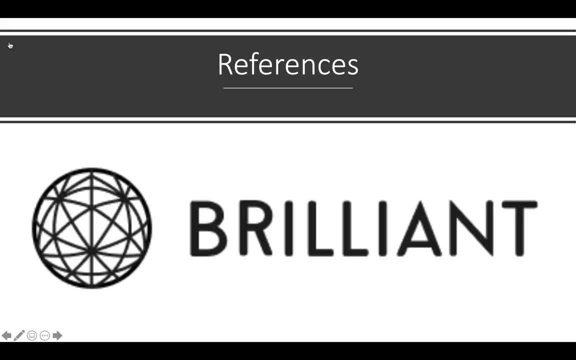 to learn more about 3d geometry or polyhedra or anything really brilliant's an excellent resource.